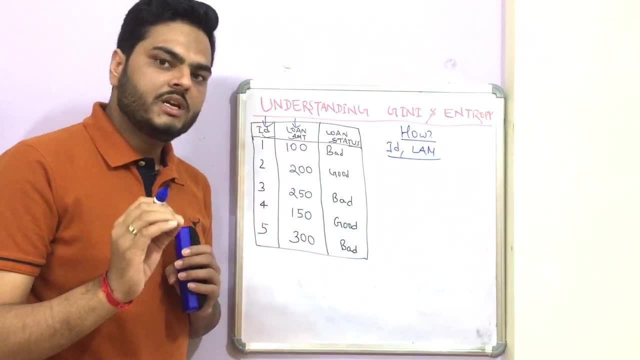 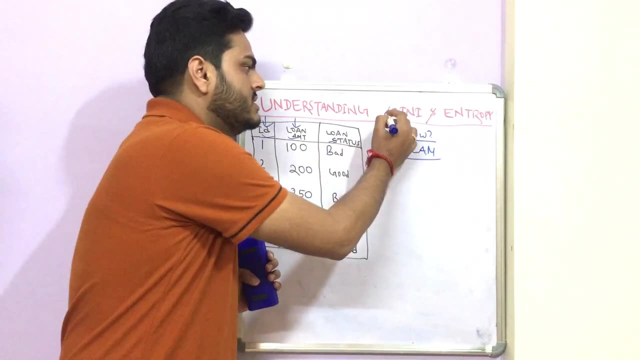 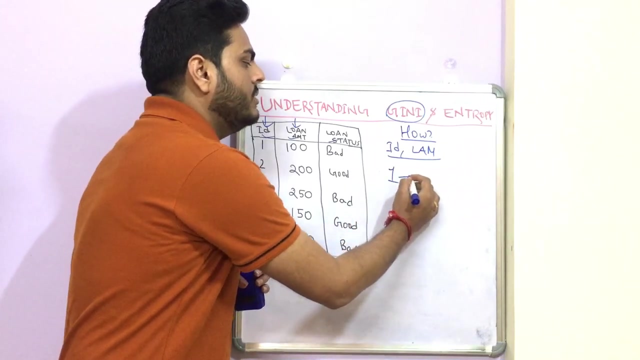 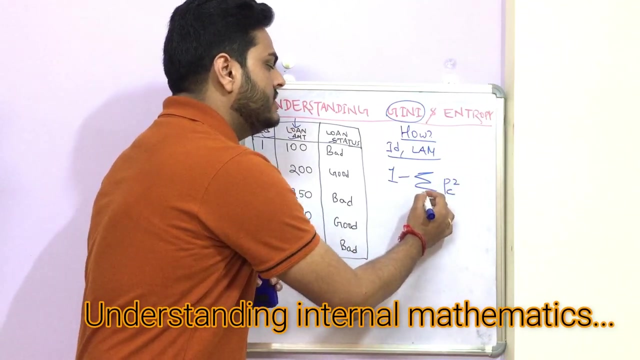 but internally the algorithm has to decide how to split and on which condition to split. So let us try understanding what is Gini index first, or Gini index. So Gini index is basically calculated by this formula: 1 minus summation of probability of c square, where c is equal to i to j. 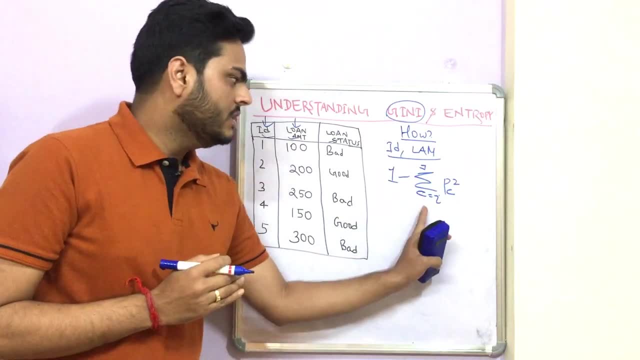 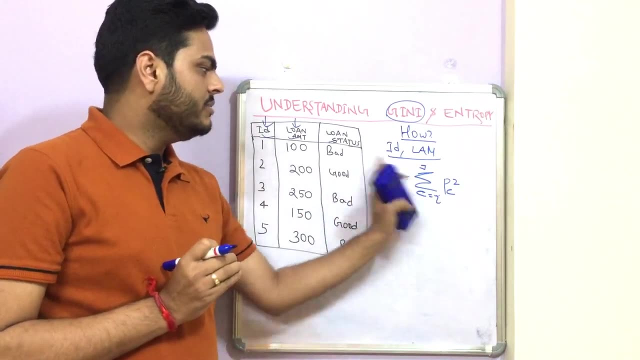 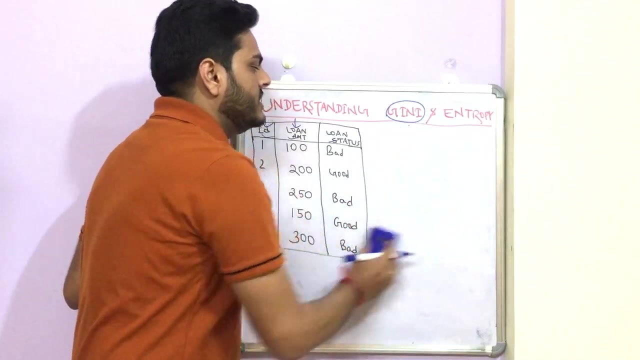 The. the meaning of this is we have to compute the probability for all the breakage that happens inside the tree. So I will give you an example and make you understand how this particular thing is calculated. Let us try understanding that. So, for example, if we say the root node, let us say 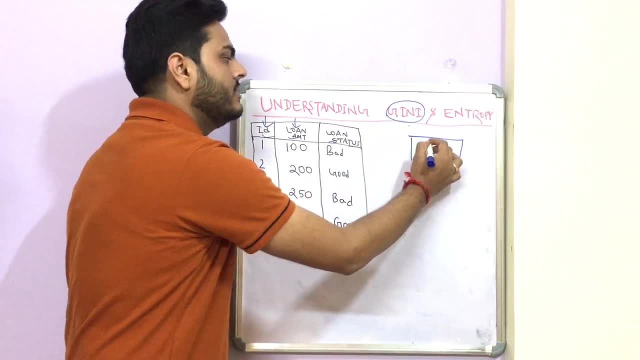 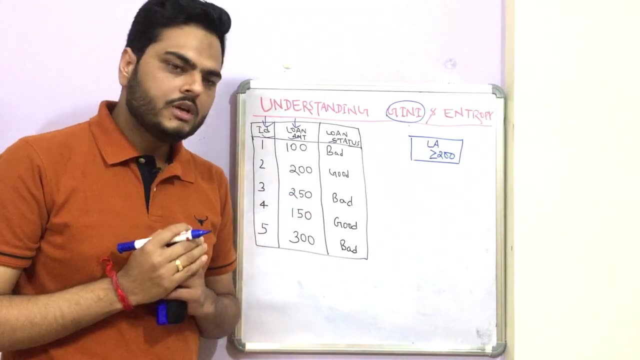 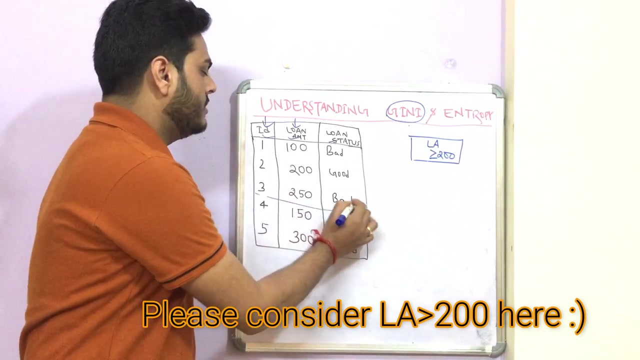 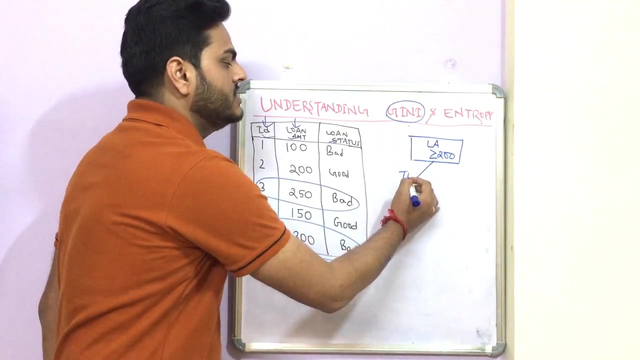 for example, the root node for this decision tree is loan amount greater than 200 or greater than equals to 200. Let us say so. how many records are greater than equals to 200 here? One record is this, other record we can see here. So let us take all these records this side, where this condition is true and for. 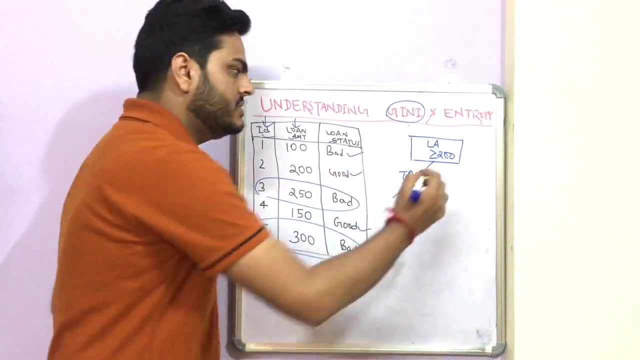 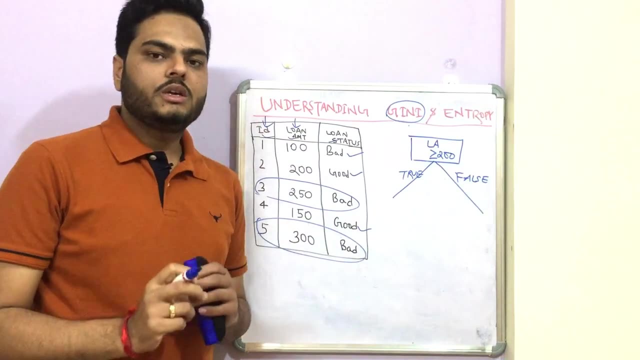 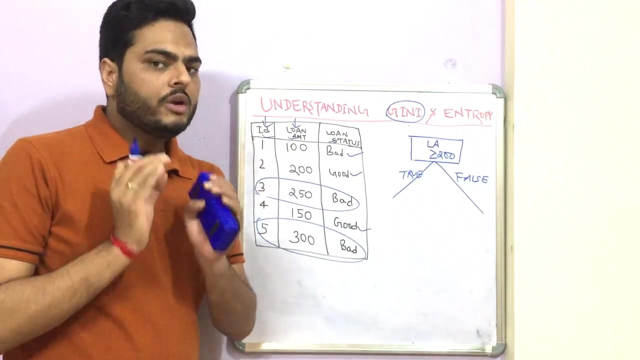 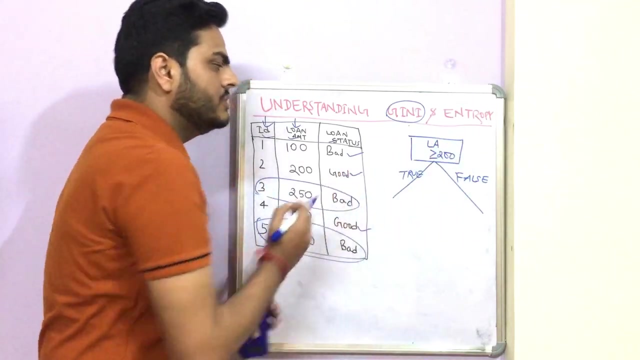 these records. this condition is false. So let us take all these records this side. So we have to actually calculate the impurity of the node. So this is an split, or we can say impurity of the split. Now what would be the best case scenario here is if we can find a condition such that all the true goes on one side. 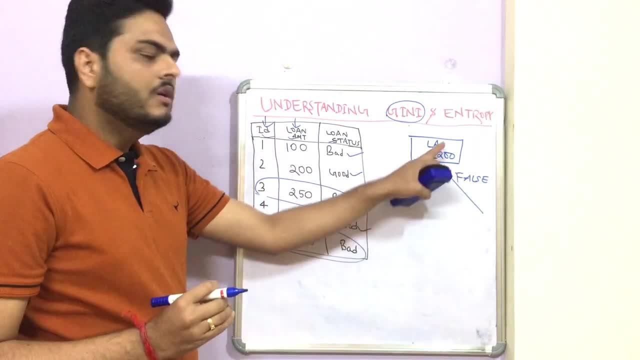 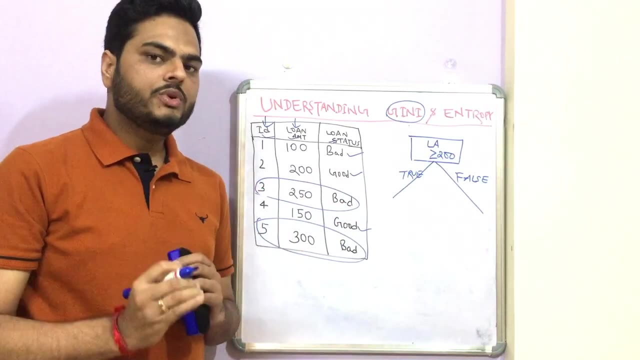 and all the false goes on one side. What I mean to say here is all the in target variable. one class comes this side and other class comes this side, If by doing something, by putting some condition, we are able to split the training data. So let us say that we are able to split the training data. 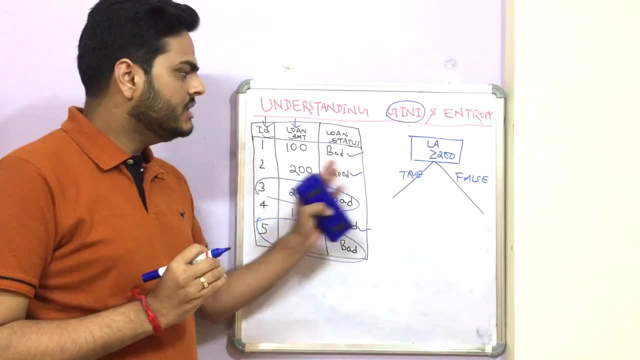 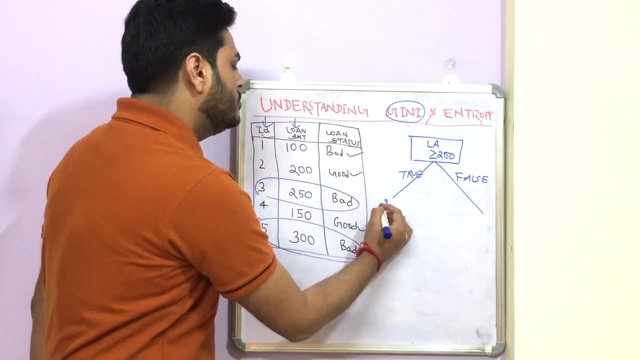 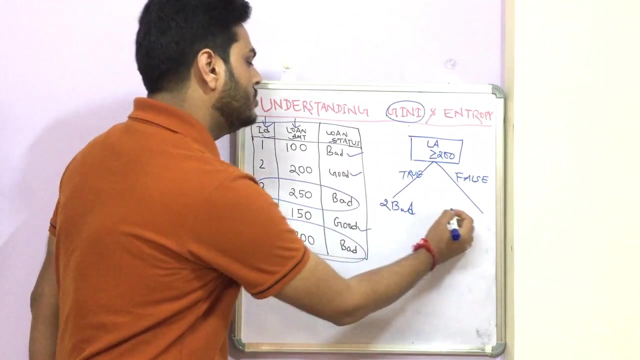 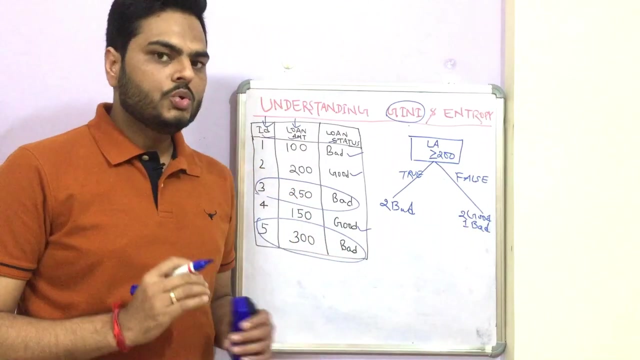 like that, Then that would be the best split. But here, when we split on this condition, then on this side of the tree we have two bad, Okay, And on this side of the tree we have two good- I'm counting here the target variable- and one bad Okay, Two good and one bad. So this is how my target variable 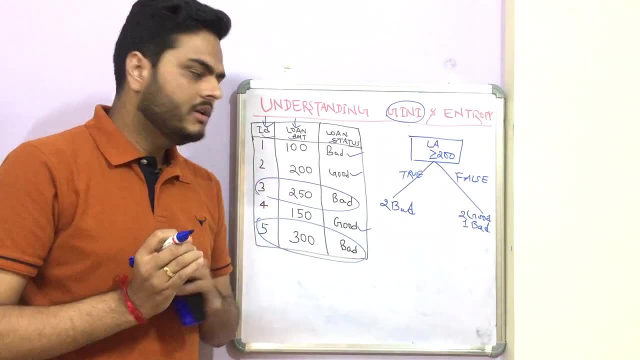 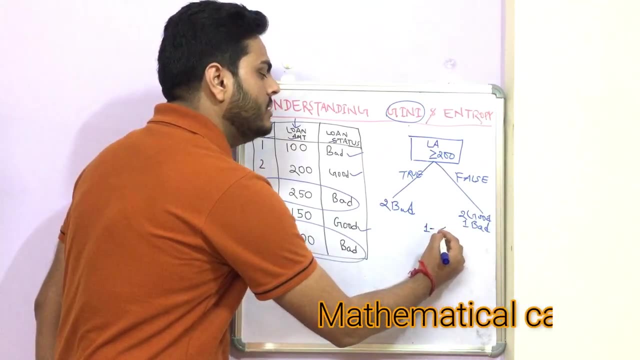 or what I intend to learn. this training is getting splitted. Now we will put this in the formula for Gini. So the formula for Gini is 1 minus summation of probability of i square. So the meaning of this. 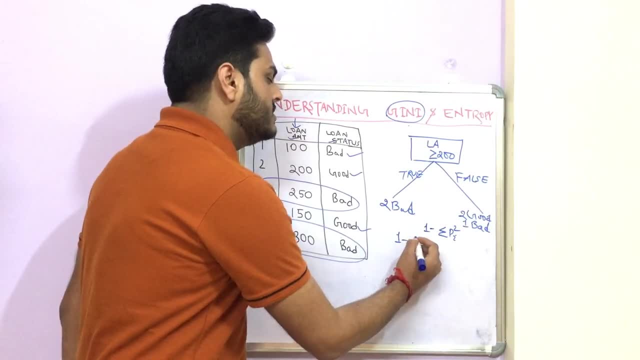 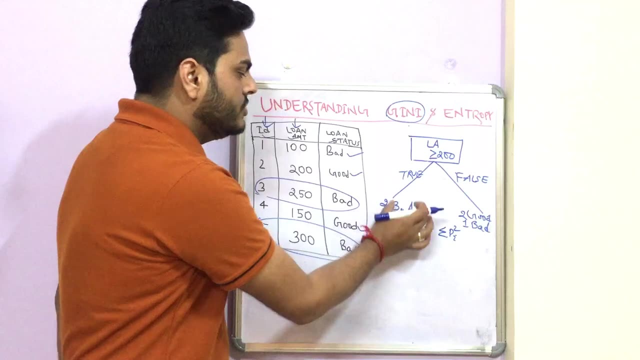 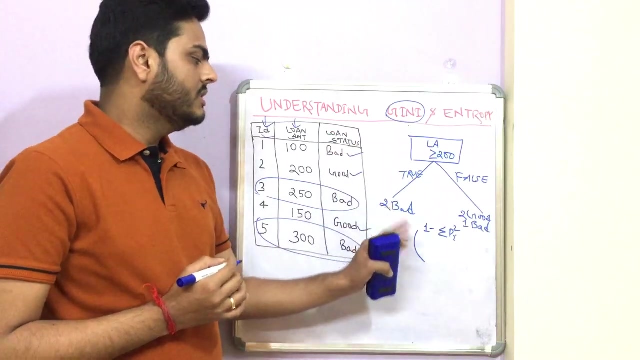 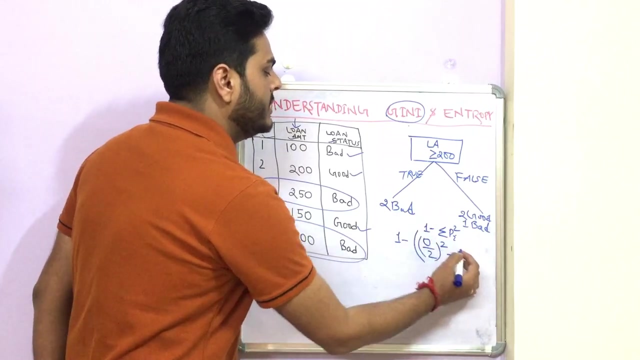 is, we will just take 1 minus probability of first. we will calculate the probability of this side of the tree. So if we come this side, then what is the probability? The probability of good class is 0 because there are 0 good classes: 0 by 2 square plus 2 by 2 square, So 2 by 2. 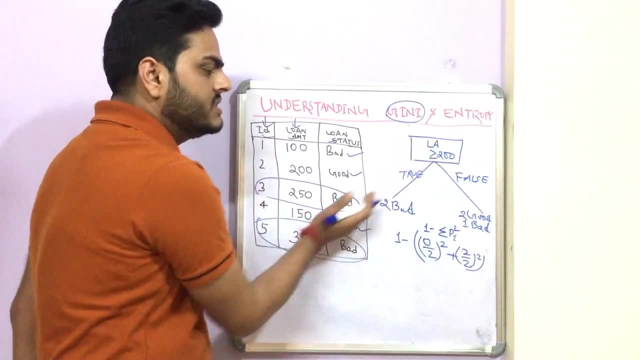 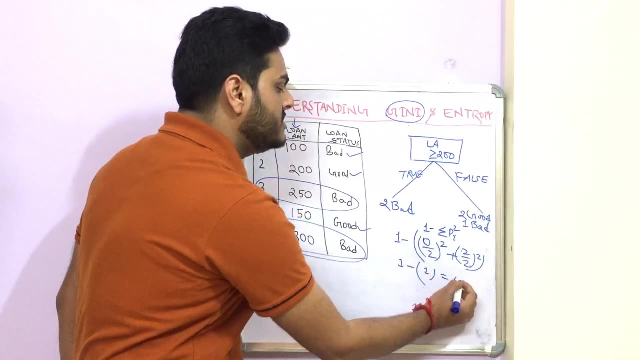 square. So this is the Gini index for this side. Now, if we compute this, it will be 1 minus, this will be 0, and this will be 1, which means 1, which means 0.. So Gini index for this side, or. 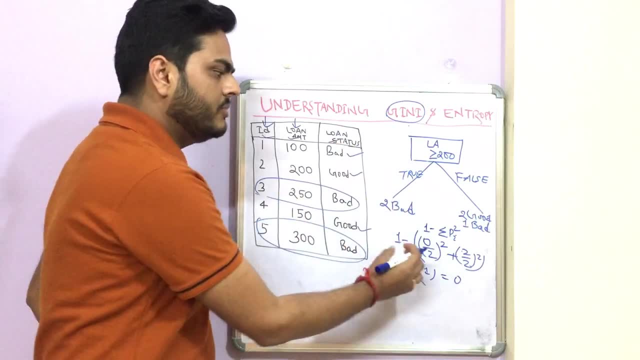 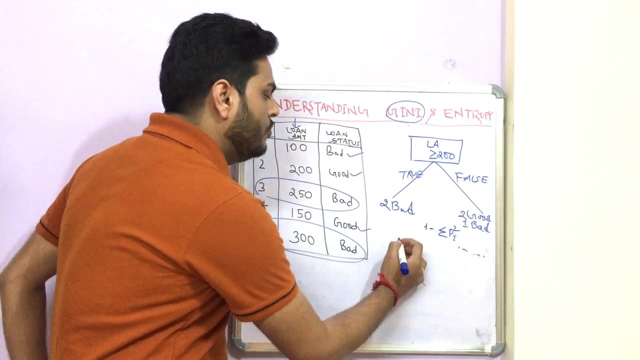 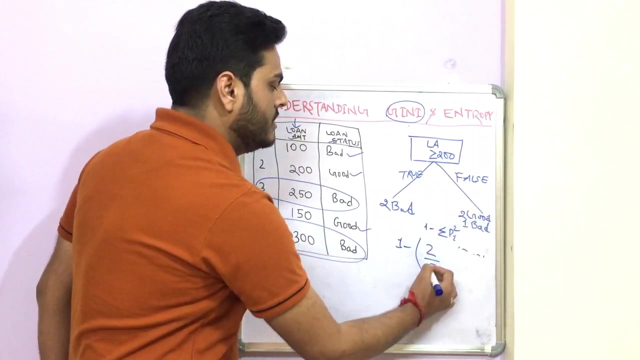 this branch of the tree will be 0. Let us put the formula for this side of the tree. So when we go for this side of the tree the Gini calculation will be 1 minus. we have to take the probability of both the class, So probability of good class 2, good classes out of 3, which 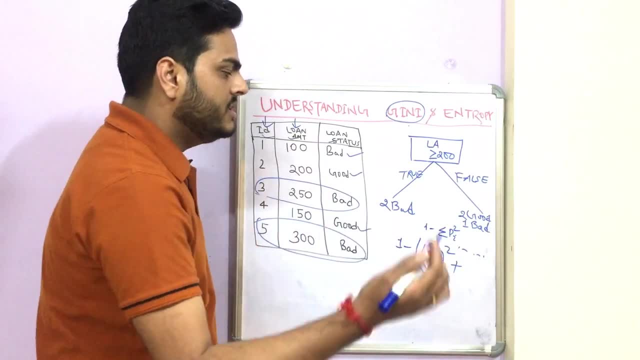 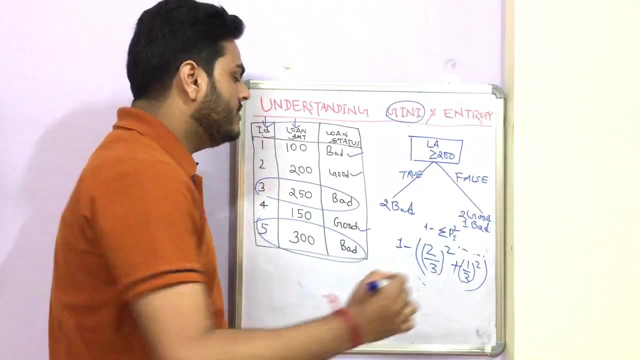 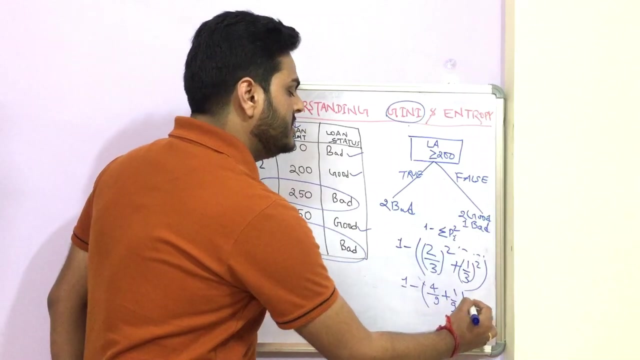 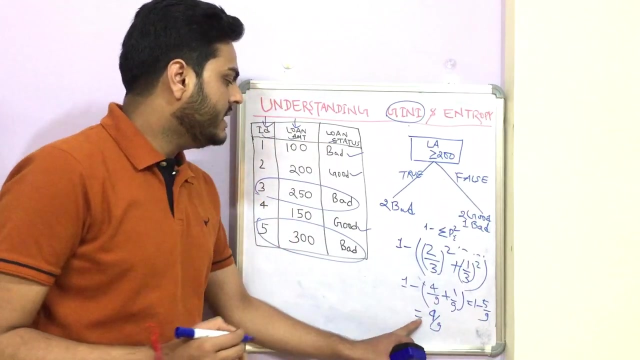 means 2 by 3 whole square plus probability of 1 by 3 square. So here how many we will have. We will have 1 minus 4 by 9 plus 1 by 9. Which means 1 minus 5 by 9, which means 4 by 9.. So 4 by 9 is the Gini index of this side and 0 is 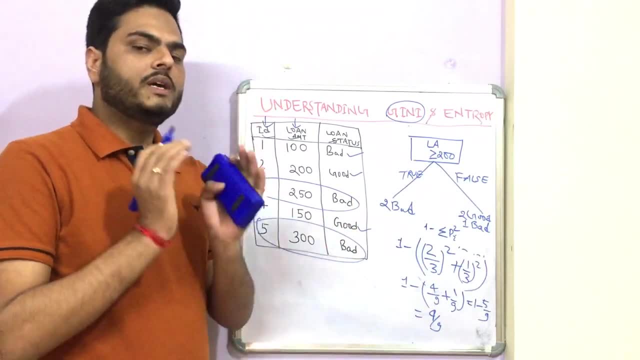 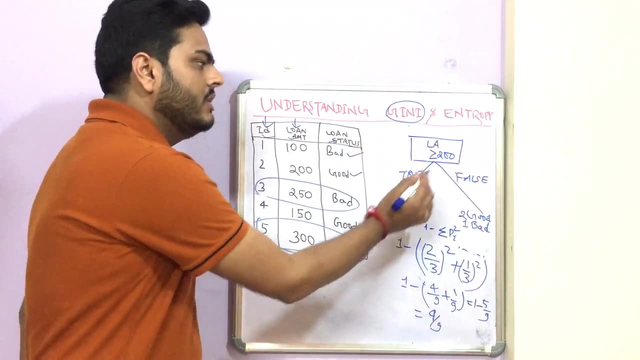 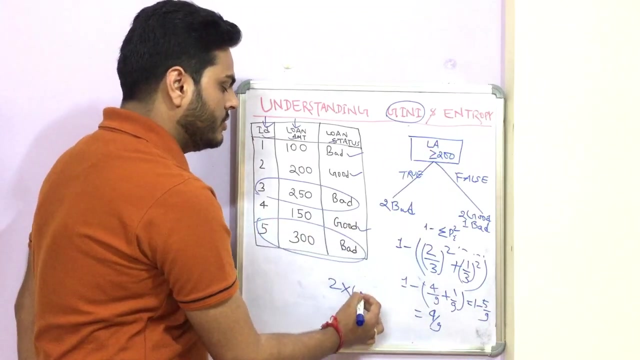 the Gini index of this side. So finally, how the final Gini index will be calculated. That is called the weighted Gini index, So that will be calculated as how many records out of 5 are on this side 2 records, So 2 into Gini index of this side, 0. 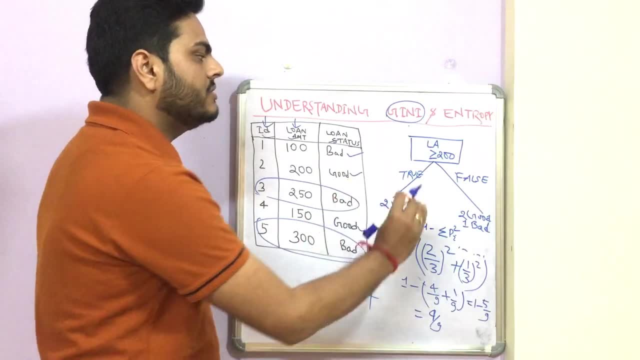 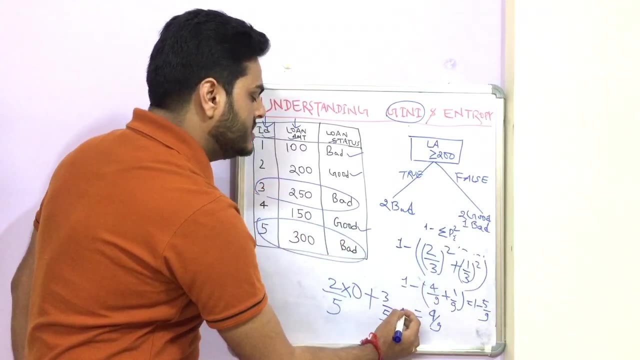 Actually 2 by 5 into 0, and how many records out of 5 went this side? 3 records, which means 3 by 5, 3 out of 5 went this side. And what is the Gini of this side? 4 by 9,, 4 by 9.. So, whatever this final 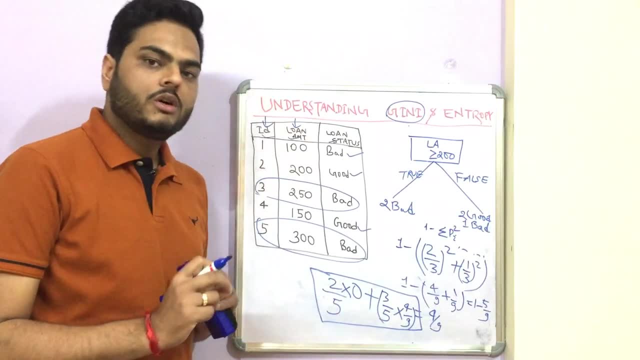 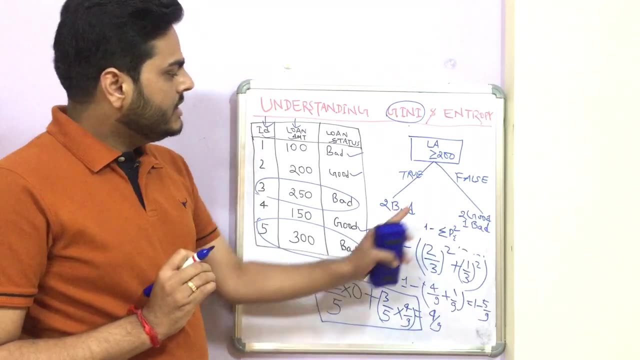 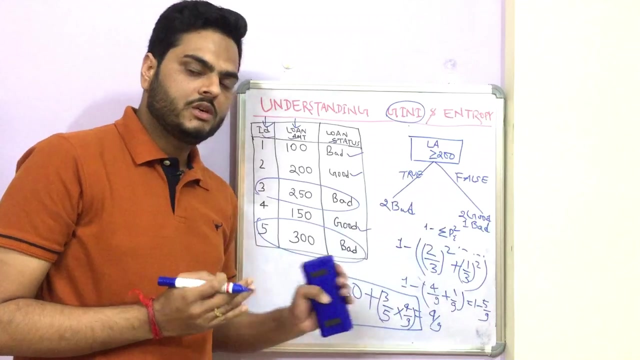 number comes, this becomes the Gini index or Gini score for this particular split. Now why Gini is 0 here is because all the classes, all the target variable, belong to the same class in this set. What happens if all bad comes this? 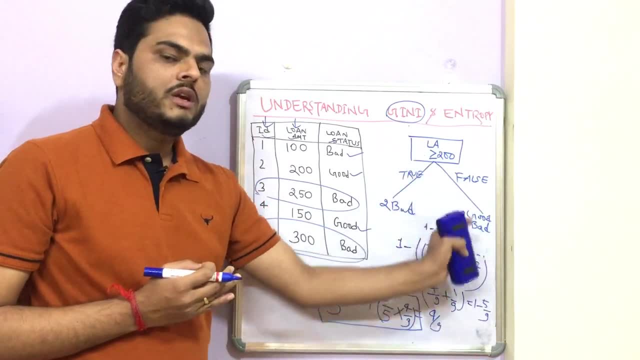 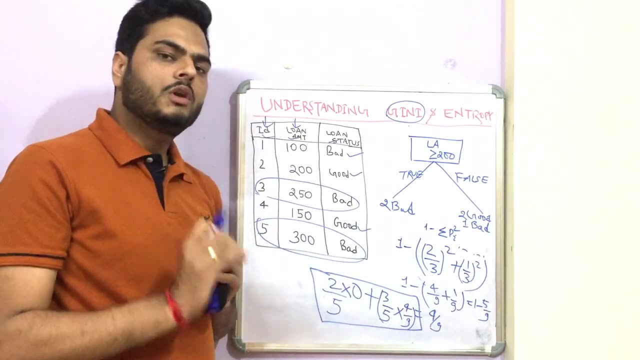 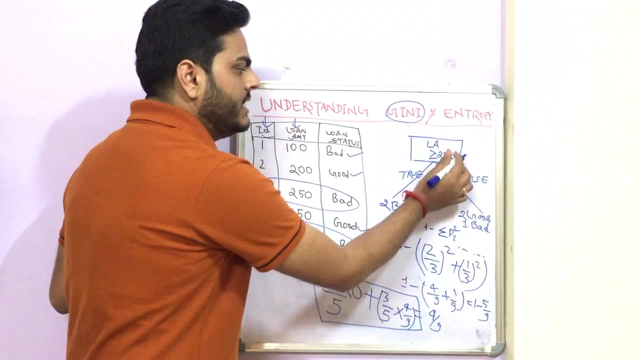 side and all good comes this side, then this side also, Gini index will be 0. In that case, the final Gini index will be 0, which is the best case scenario. So Gini index will always range between 0 to 1.. Apart from that, let us say, in place of this L, a greater than equals to 200, if we take 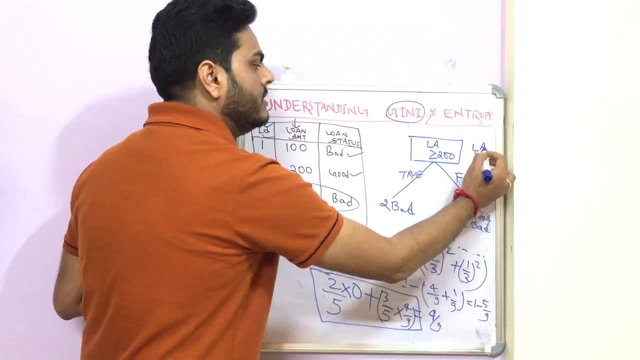 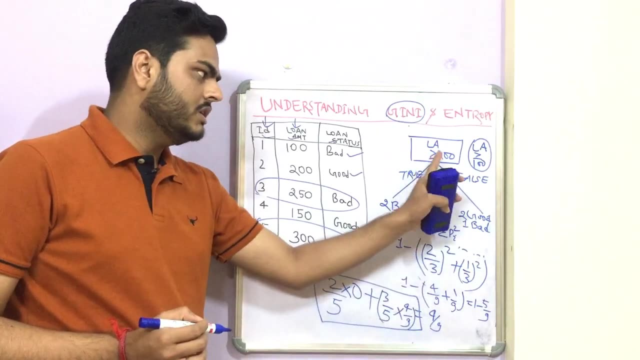 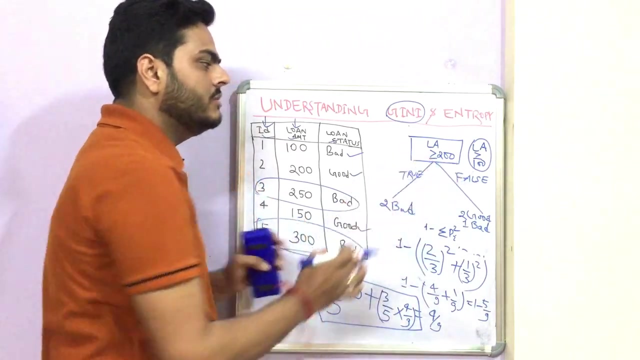 another condition. let us say L, a greater than equals to 100.. We compute Gini index like this, like the way we calculated for this condition, and what will happen inside the algorithm is algorithm will compare the Gini index for this condition and this condition not only for a. 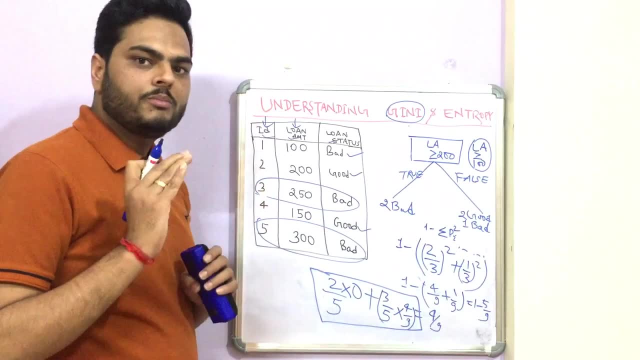 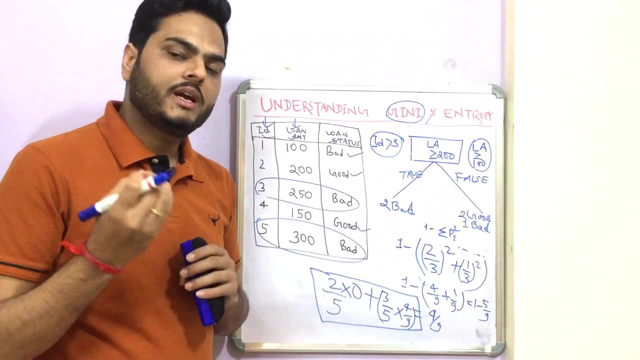 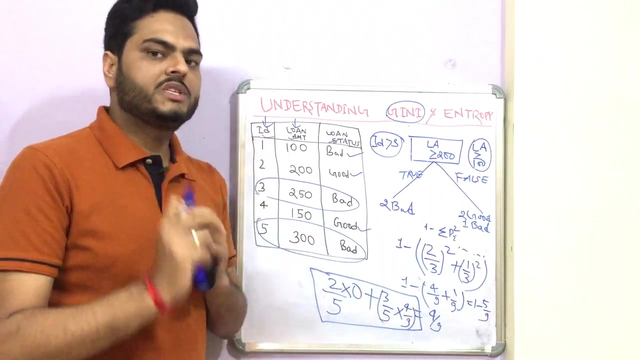 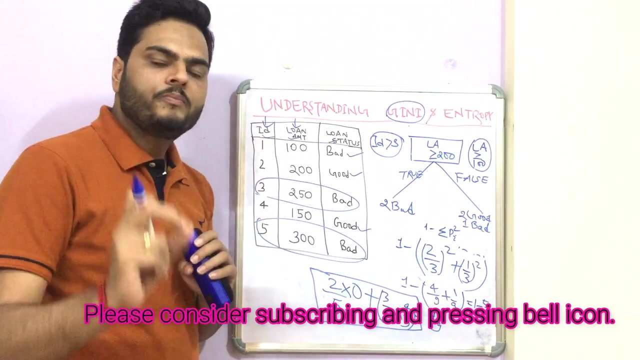 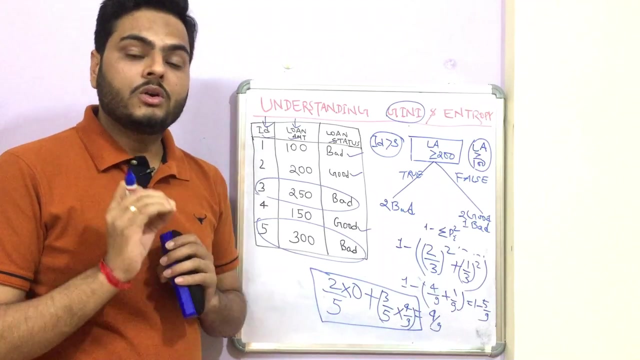 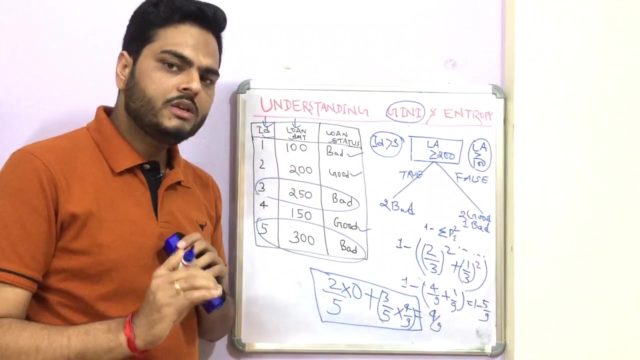 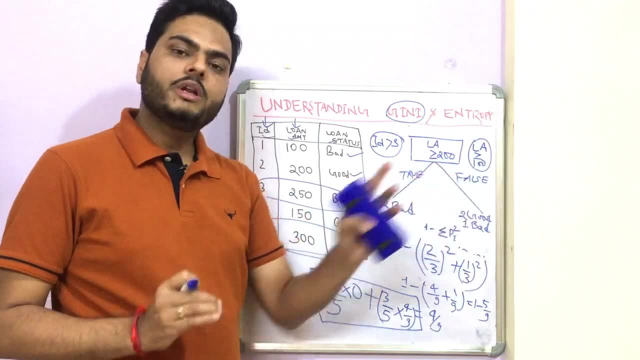 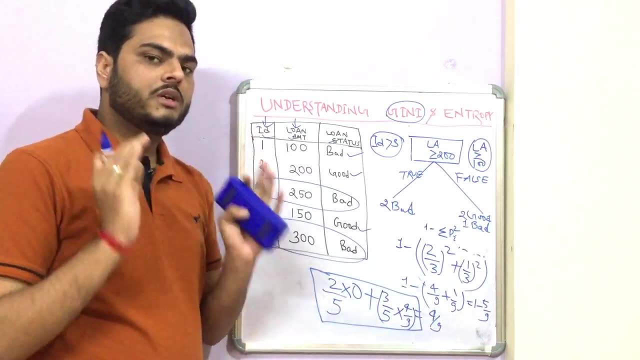 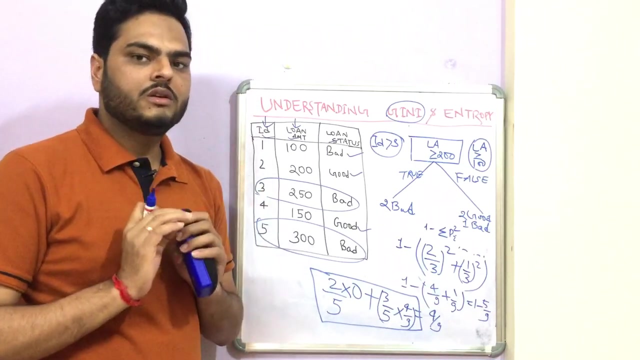 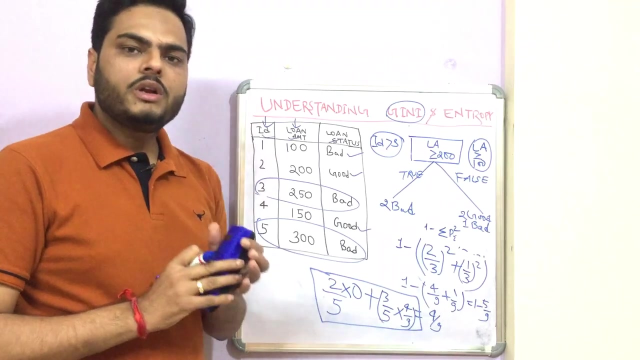 guinea index from all the available condition. how guinea index will be calculated? like this: minimum guinea index from all the required, all the available columns and conditions, wherever it finds the minimum value, that will be selected as the criteria for the split. okay, so guinea is nothing but a selection criteria, or tree split criteria when we call decision tree. 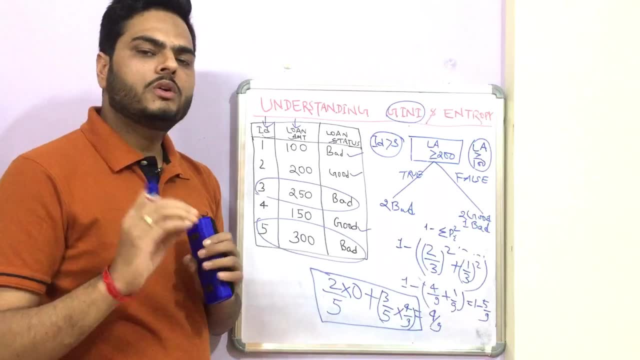 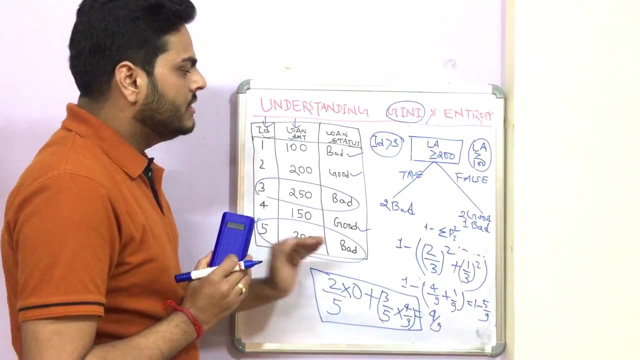 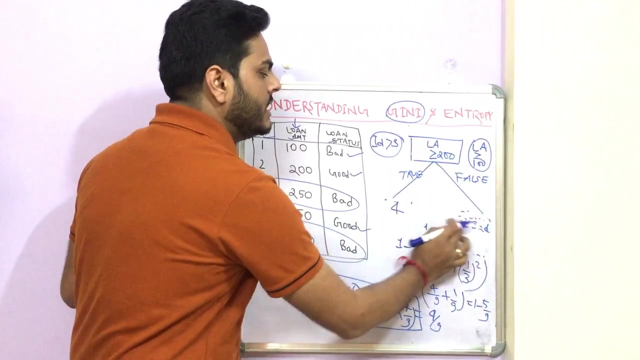 algorithm. we just say criteria is equal to guinea or in some languages, guinea is the default splitting criteria for the tree. imagine a situation where in this there are four records and in this there are also four records- okay and two, good here and two, bad here and two. 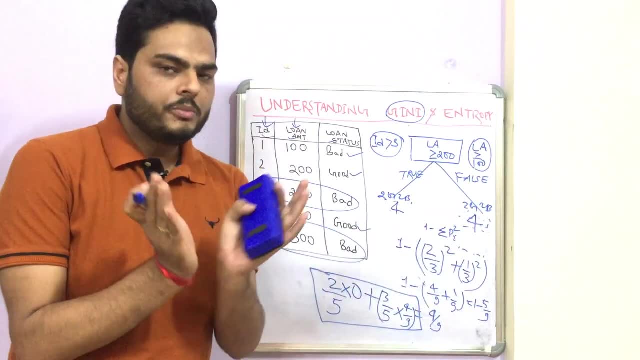 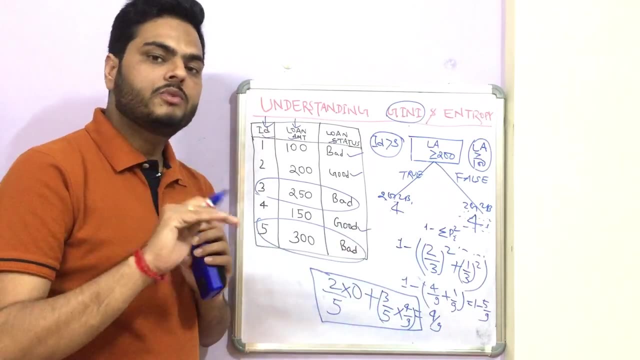 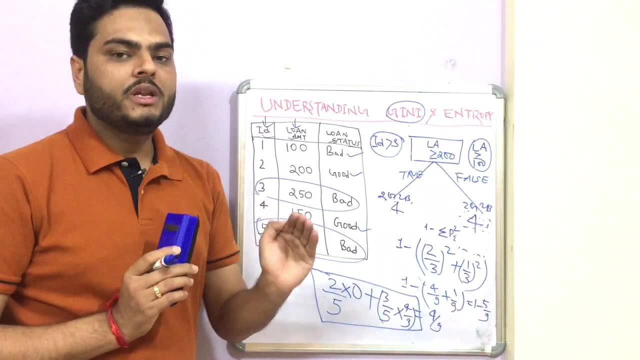 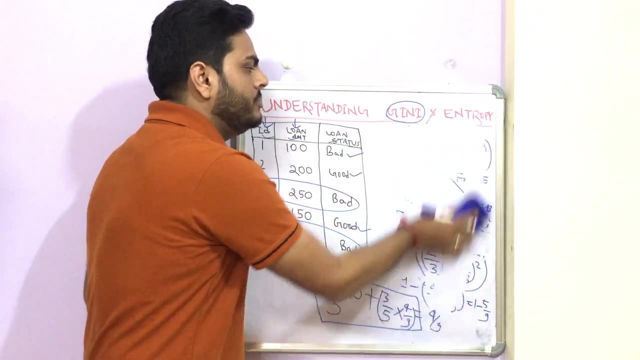 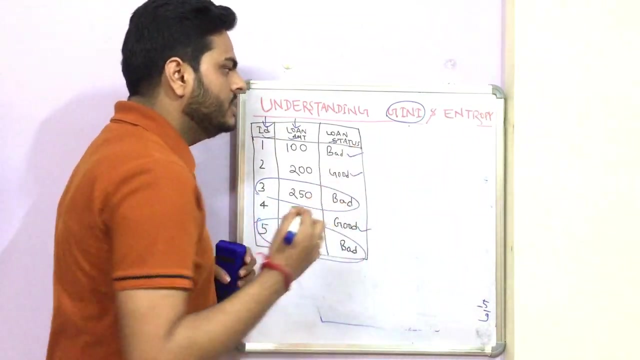 how guinea index is calculated and how minimum guinea index is chosen for the tree splitting. okay, there is another splitting criteria called entropy, commonly known as information gain. okay, so when we call a decision tree algorithm, as i told you in some of the languages you just say: 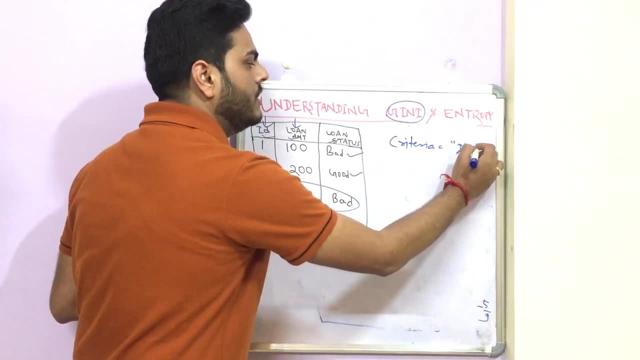 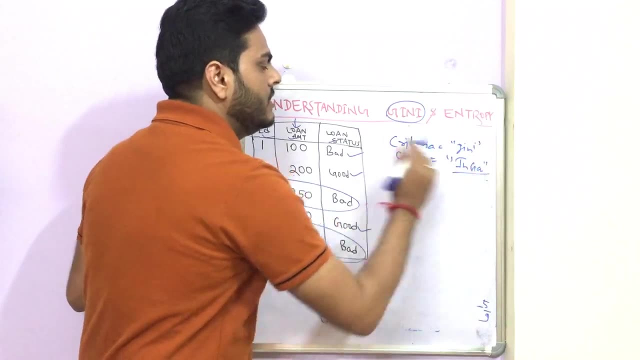 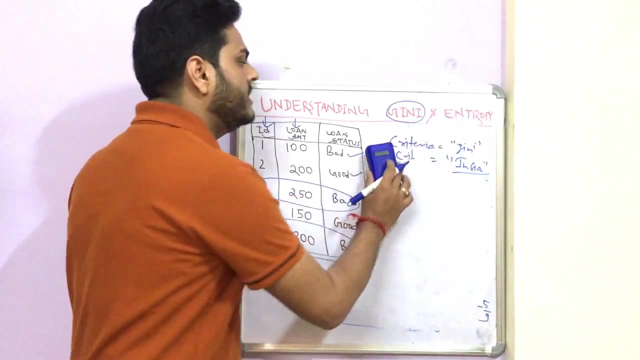 criteria is equal to guinea, okay. or you can say: criteria is equal to entropy or information gain. okay, information gain. but in some of the languages, as i told, this is the default. you know splitting criteria. so how is entropy different from guinea index? just the formula, why it is different. what is the formula? 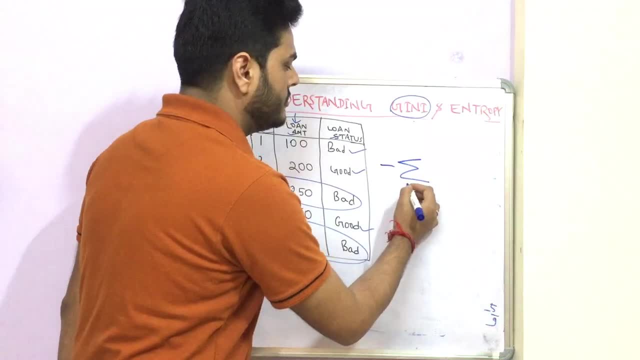 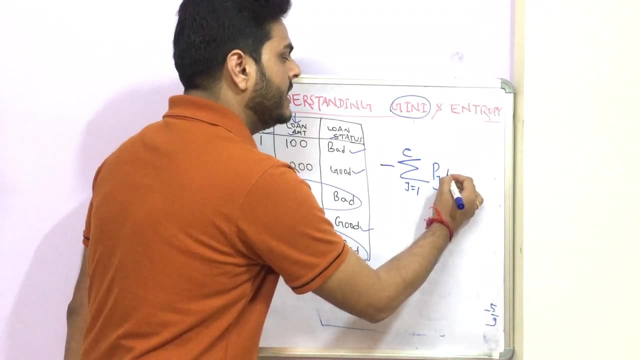 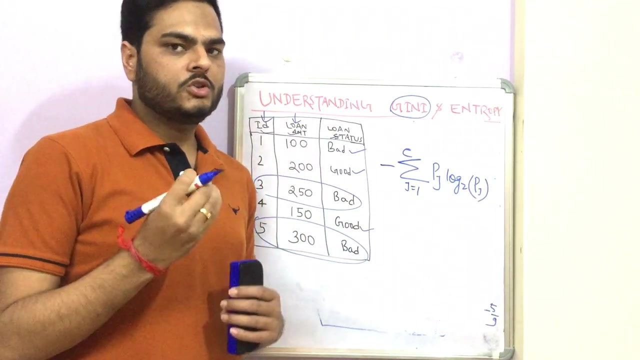 for entropy minus summation of j is equal to 1 to c probability of j multiplied by log base 2 probability of j. so this is the only difference between guinea and entropy. the formula for entropy, or information gain, is this what you can see on the screen. 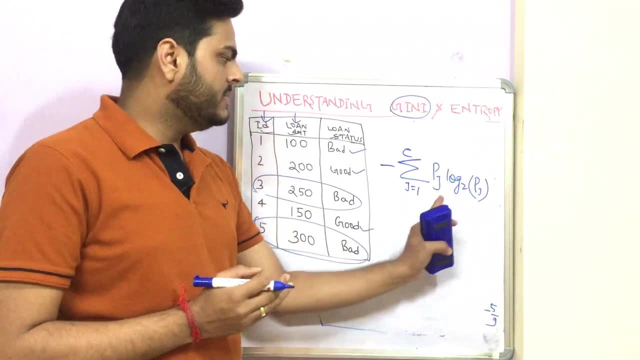 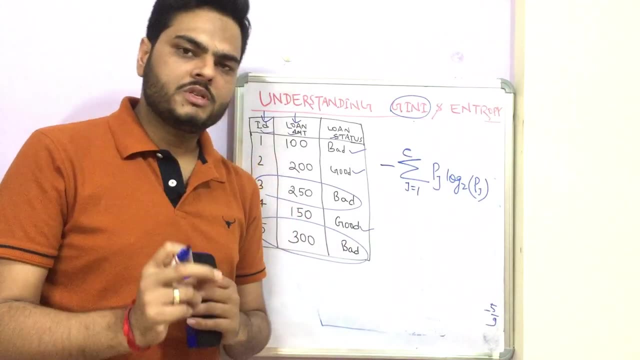 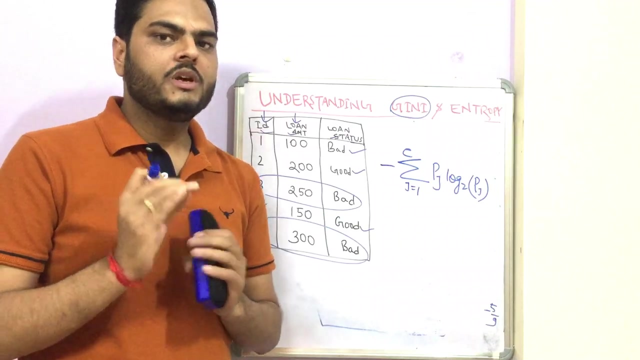 and again, similarly, the way we calculated probabilities. probabilities will be calculated and information gain will be computed and then, wherever the lowest information gain occurs, that particular condition will be selected as the condition for splitting of the tree. so that is how guinea and entropy works on the condition wise where to split the tree. 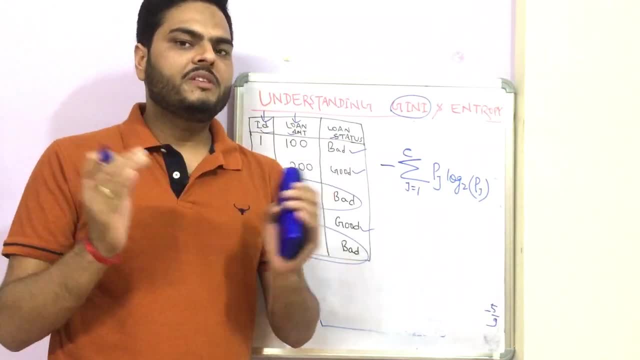 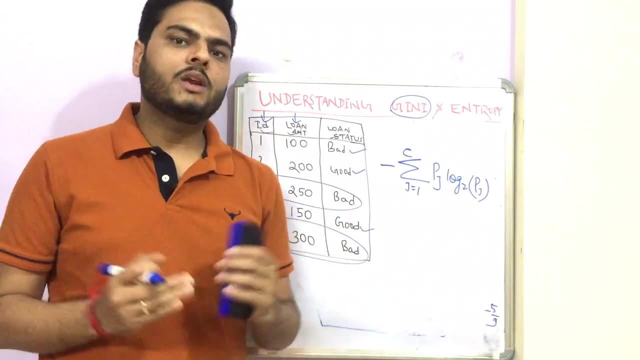 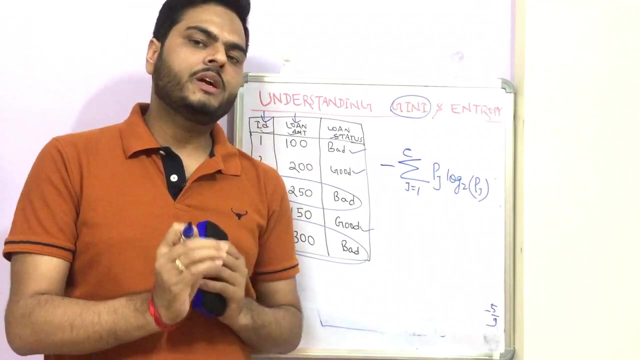 now to ask what to use when. so, basically, guinea is a little faster because the calculation is little simpler. in entropy you have log function and hence calculation sometimes takes more time, but end of it, it's your data and it's your you know model that decides which of these two criteria.